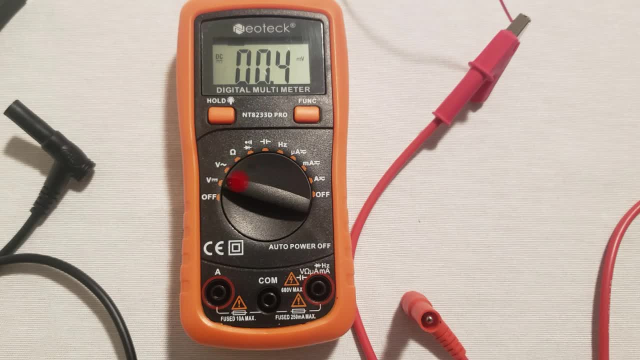 voltage, represented by the little sine wave that you see there. If you want to measure the resistance, use this setting. If you want to measure continuity or the functionality of a diode, use this Here. if you want to measure the capacitance of a capacitor, this is where you want to put your. dial at And this is for frequency for an AC signal, And if you want to measure small amounts of current in microamps or milliamps, you could use the setting here. And this is for a DC current or AC current. DC current stands for direct current which flows in one direction: AC current. 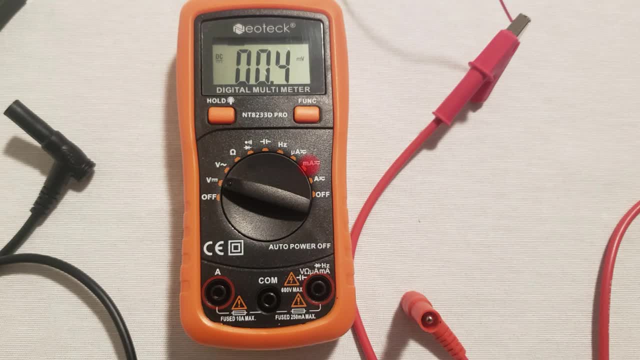 stands for alternating current which flows in both directions. And, of course, if you're using this setting, make sure the red test lead is on the left. If you're using these two settings here, make sure the red test lead is on the right. One thing I do like about this particular multimeter: 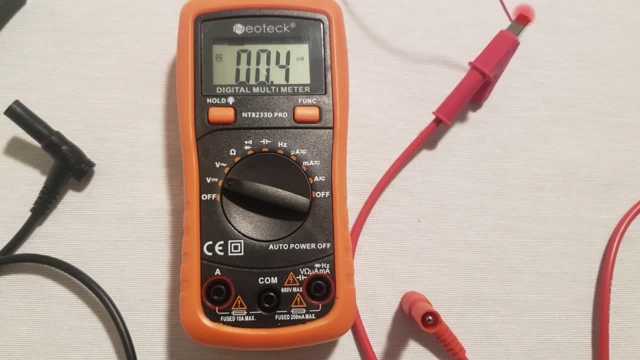 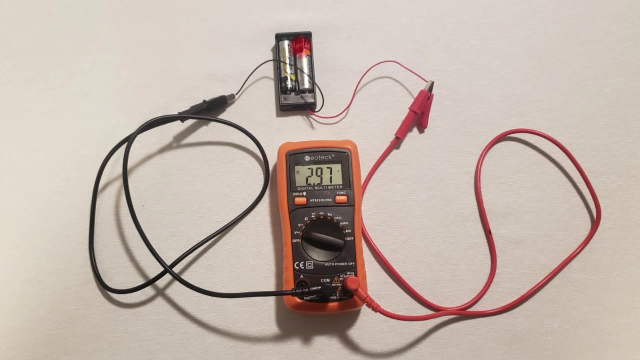 are the test leads, because they have the clamps where you can clamp it down to whatever device you're trying to measure or whatever component you want to have measured. So that's one useful feature of this particular multimeter. In this picture I'm measuring the voltage of these two. 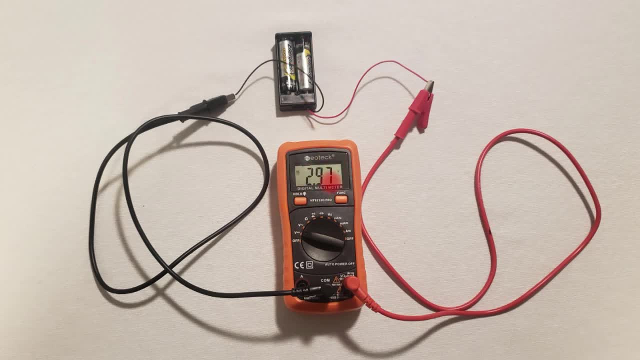 AA batteries, which is close to 3 volts. As you can see, it's reading 2.97.. You want to connect to the black wire of the battery and the red lead to the red wire of the battery And make sure the 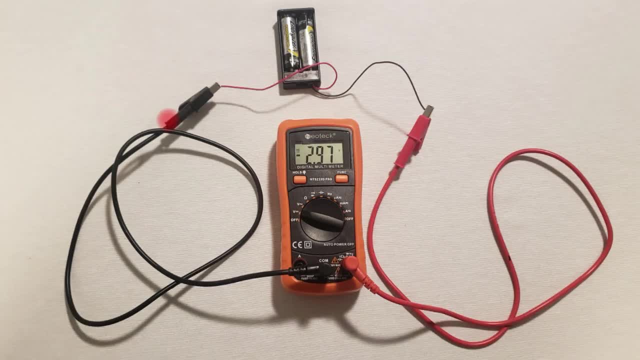 setting is at DC voltage. Now notice what happens when you reverse the connection. Here I have the red wire attached to the black test lead and the black wire attached to the red test lead. Notice that we have a negative sign displayed in the multimeter. So it simply means that the connection 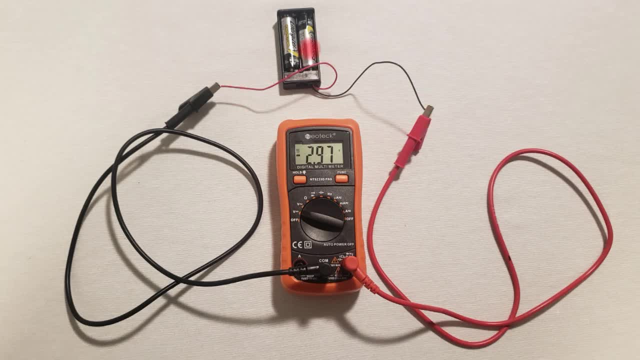 has been reversed, So this is a good way to determine the polarity of the battery. If you see the negative sign, you're going to have a negative sign displayed in the multimeter, So just reverse the connection. If there's no negative sign, then you have it connected the right way. 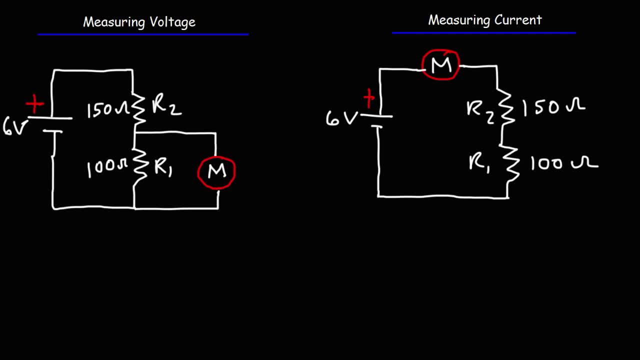 Two common values that you'll often need to measure when using a multimeter are voltage and current, So it's important to know how to measure these things properly. When measuring voltage, you're going to measure it across an element like a resistor, So you want. 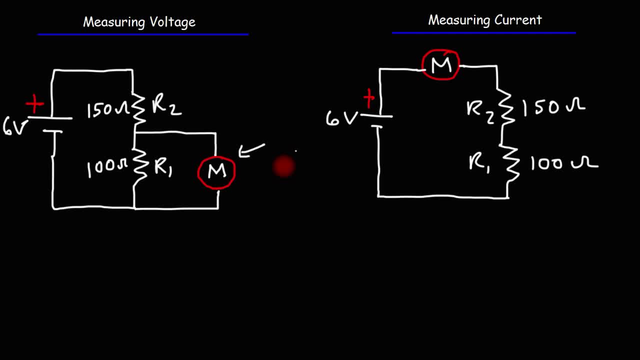 to connect your meter across the resistor, not through it. So that is, you want to connect the meter parallel to the resistor, So you want to connect the meter parallel to the resistor. So you want to connect the meter parallel to a resistor In order to measure current, the current. 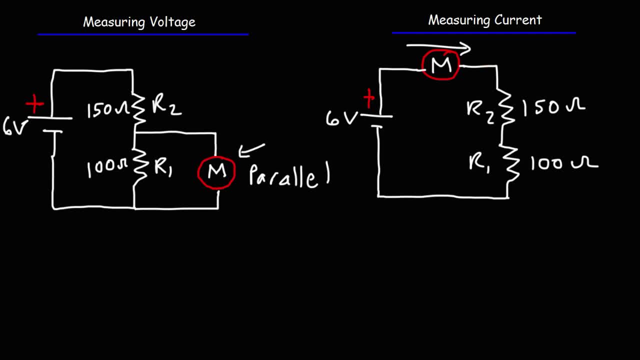 has to flow through the meter, not across it. So you want to connect the meter in series with the resistors, And so that's the difference between measuring voltage and current. You measure voltage across an element that is in parallel with the element, And to measure current, the current has. 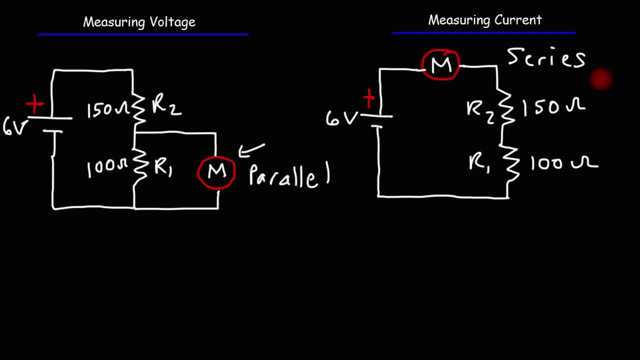 to flow through the meter. So you connect the meter in series with the circuit. Now here's a math for this question for you. What do you think will be the voltage that the meter will read across R1?? How do you find the answer? Well, we need to use something called Ohm's law. 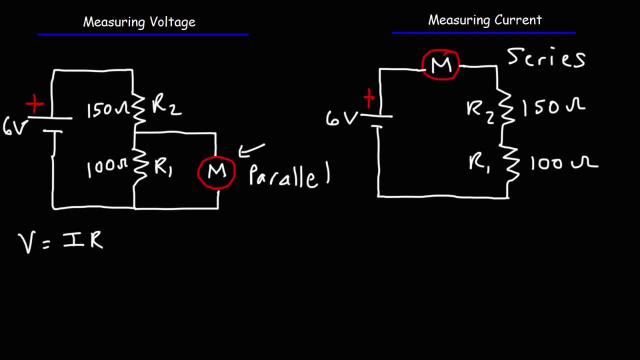 Voltage is equal to current times resistance. Now we have two resistors in series, so the total resistance is going to be R1 plus R2.. That's 150 plus 100, so that's 250 ohms. And we have a 6-volt battery across those two resistors. so, using Ohm's law, V equals IR. 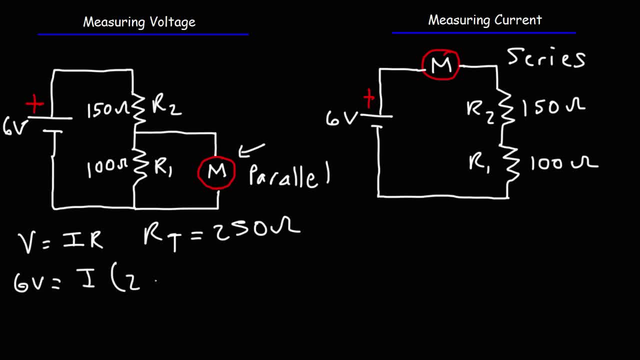 we have a voltage of 6 and a resistance of 250.. So dividing both sides by 250,, the current flowing in the circuit is going to be 6 divided by 250, and so the current is 0.024 amps. 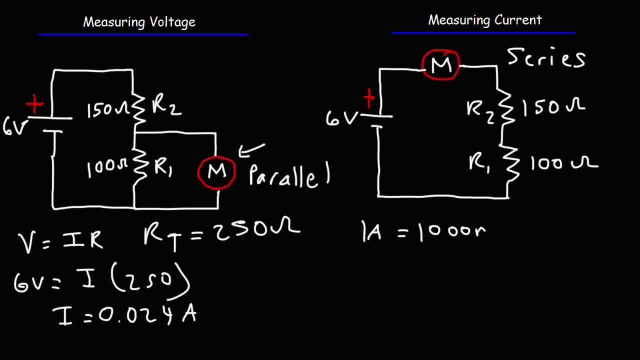 One amp is equal to 1,000 milliamps. So multiplying 0.024 times 1,000 gives us a current of 24 milliamps. Now for the circuit on the right. that's what the meter is going to be measuring. It's going. 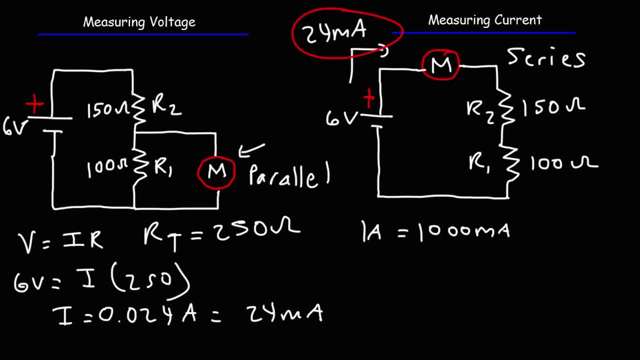 to measure a current of 24 milliamps. Now, going back to the circuit on the left, the current that's flowing in that circuit is also 24 milliamps, because the voltage of the battery is the same and the value of the two resistors are the same. 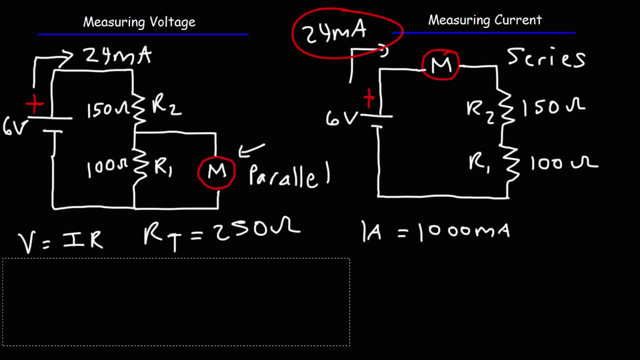 So to calculate the voltage across R1, we can once again use Ohm's law. V equals IR, So the voltage across R1 is going to be the current that's flowing through it, That's 24 milliamps, which is 0.024 amps times the resistance of R1, which is 100 ohms. 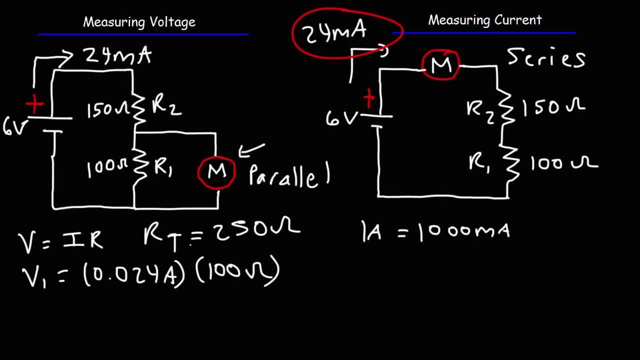 So 100 times 0.024.. So the voltage across R1, as read by the multimeter, will be 2.024.. will be 2.4 volts. So that's how you can calculate it. There's also another method that you could use. 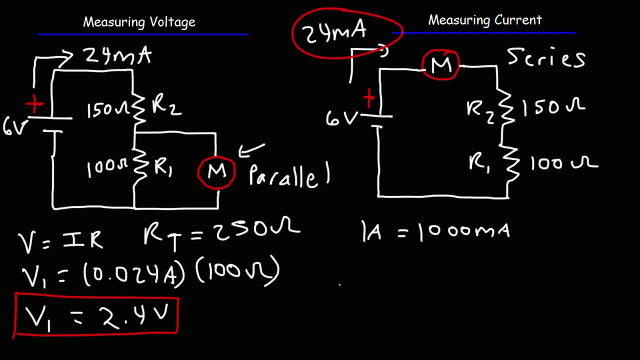 because this circuit forms a voltage divider circuit. You could use this formula: V1 is going to be equal to R1 over R1 plus R2 times the voltage of the battery. So R1 is 100.. R1 plus R2, that's. 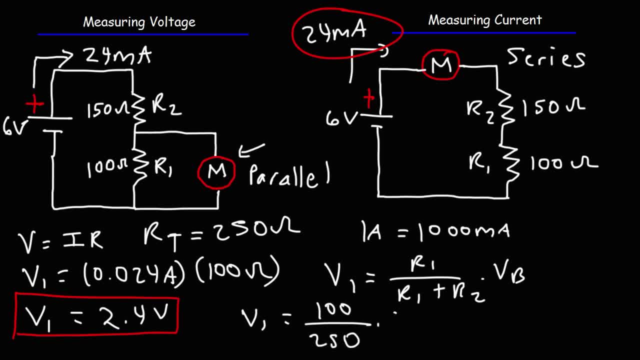 100 plus 150, that's 250, times 6 volts. So 6 times 100 is 600 divided by 250.. That's going to give you 2.4 volts as well. So that's another way in which you can calculate the voltage across R1.. 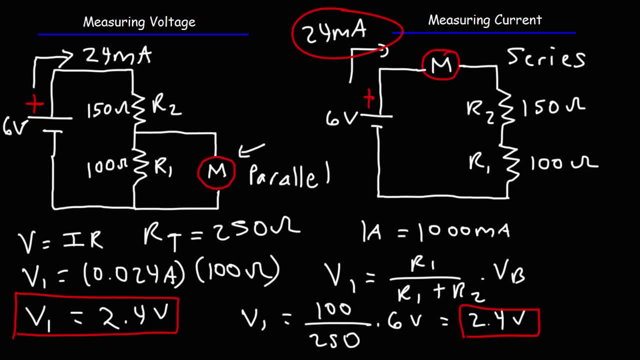 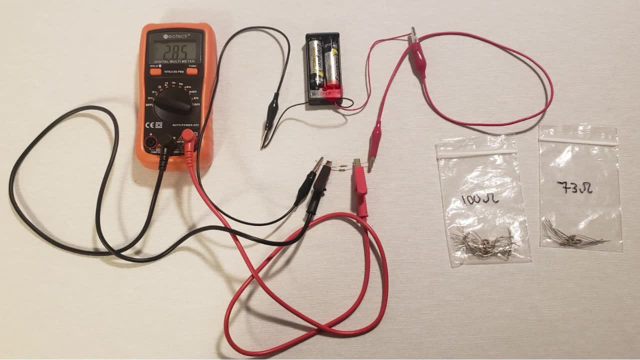 But now you know how to measure the voltage across a resistor and how to measure the current flowing in a circuit, So just keep these things in mind. So here is a picture That shows how to measure the voltage across a resistor Current that is conventional current. 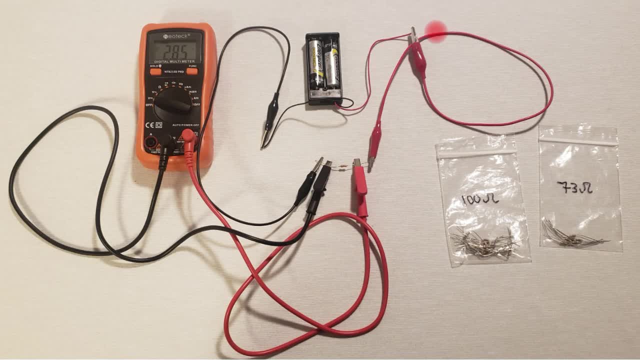 will flow from the positive terminal of the battery through the red wire, through the 100 ohm resistor, through the black wire, back to the battery. Electrons actually flow in the opposite direction. To measure the voltage across the resistor, simply connect the black test lead. 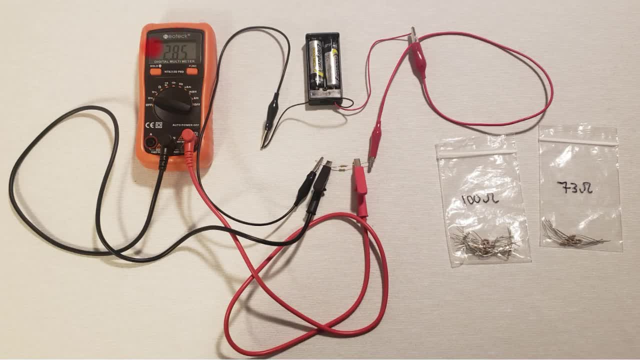 and the red test lead across the resistor And, as you could see, we have a voltage of 2.85 volts, which is a little bit less than the voltage across the resistor. So we're going to measure the voltage across the resistor. 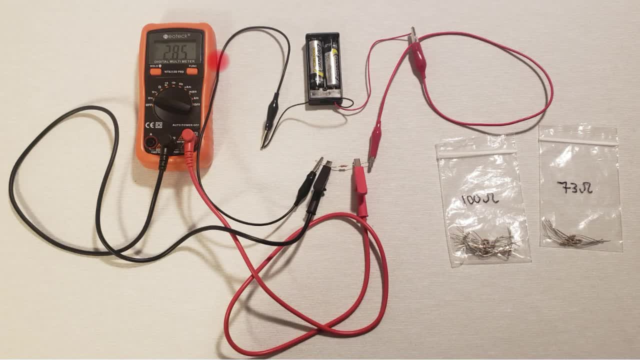 The open circuit voltage of the battery that you saw in the earlier picture, which was about 2.97 volts. Whenever you connect the battery to a resistor, that resistor is going to draw energy away from the battery, giving it a slight voltage drop. If I were to use a 10 kilo ohm resistor, 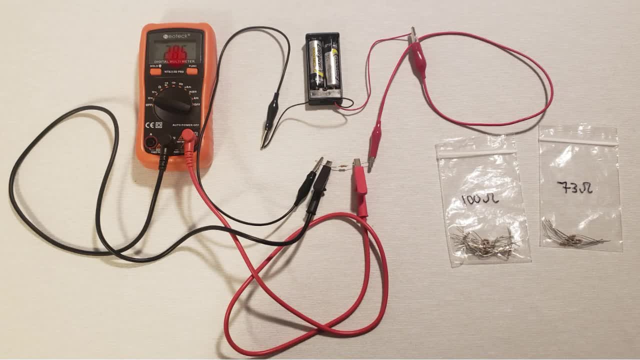 the voltage across the battery would be like 2.97, maybe 2.96.. It wouldn't change much. But when you use a lower resistor value, like 100 ohms or even 10 ohms, the voltage is going to drop more because it's drawn more current away from the battery. 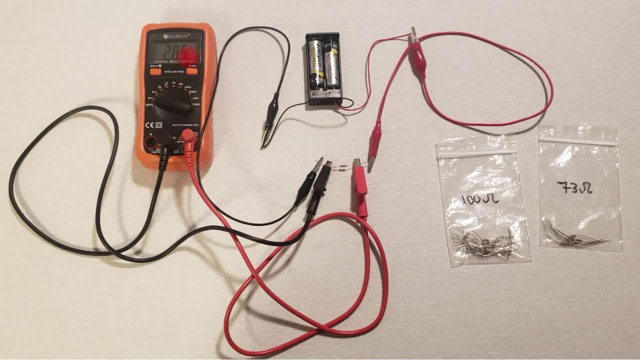 So if I were to use a 10 ohm resistor, the voltage across the resistor will be a lot less than 2.85.. So just keep that in mind. Whenever energy is drawn from a battery, the voltage across the battery will decrease. The more current that you draw away from the battery, the greater the 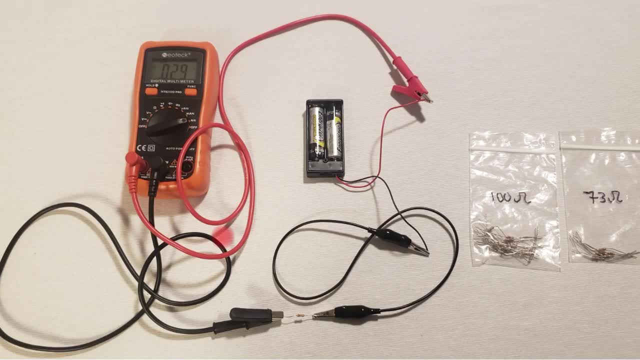 decrease in voltage across the battery will be. Here is an example of how to measure the current flowing in a circuit. So notice that the multimeter is connected in series with the resistor and the battery. So conventional current will flow from the positive terminal battery through the red test lead into 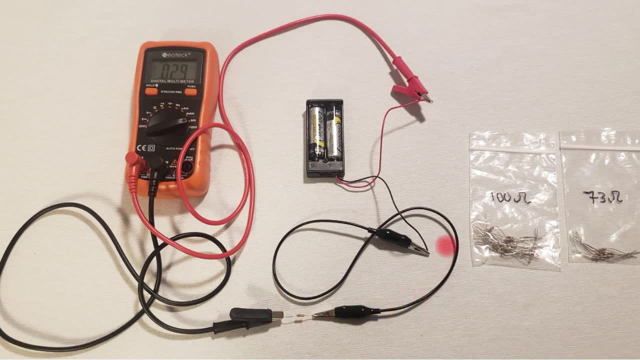 the multimeter out of the black test, lead through the resistor and then through this black wire back to the battery. So the multimeter is connected as part of the circuit. It's in series with the circuit. So you want the current to flow through the multimeter And we can see. 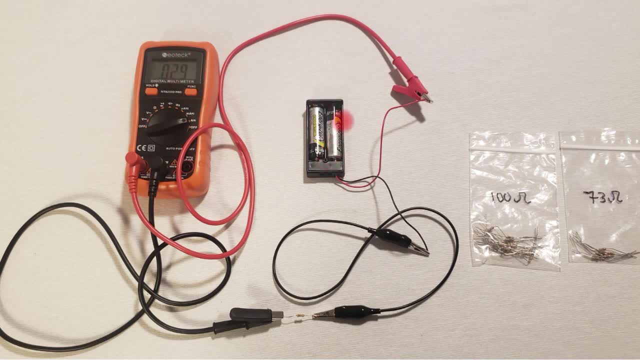 that the reading is accurate: 0.029 amps. We know the voltage of the battery is 2.9 volts And so if you take 2.9 volts divided by the 100 ohm resistor, you're going to get a current of 0.029 amps. 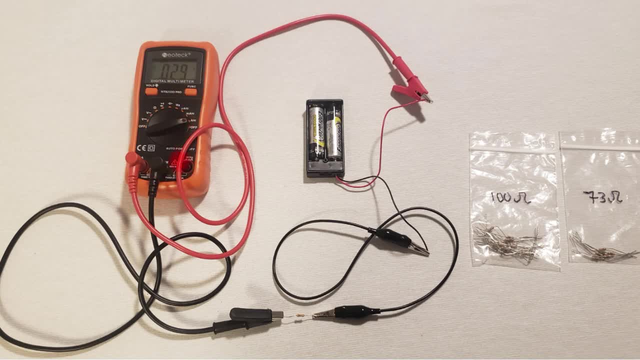 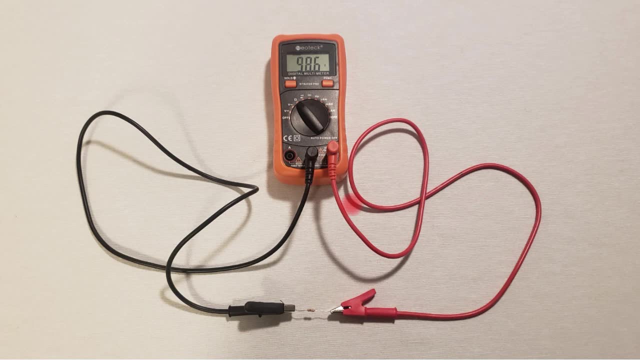 Now I could use the milliamp setting, but I'll have to put the red test lead here and it would give me a reading of 29 milliamps. Now, the next function that we're going to talk about is how to measure the resistance of a resistor, So make sure the red test lead is. 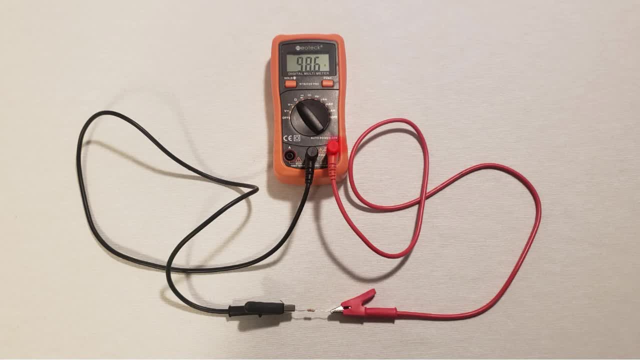 connected to the right side, where you have the resistance symbol, and turn it down to the resistance symbol, which is the ohms symbol, and just connect the two test leads across the resistor And for the 100 ohm resistor we have an actual value of 98.6 ohms. So these resistors 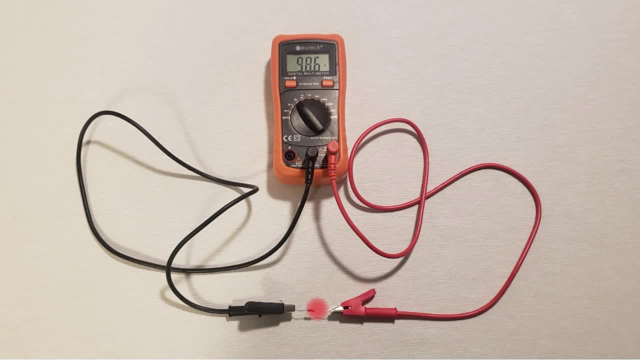 are not perfect, so to speak. Even though it says it's a 100 ohm resistor, it's going to vary from 100 ohms, It could be 101,, it could be 99, but it's going to be close to 100. But that's how. 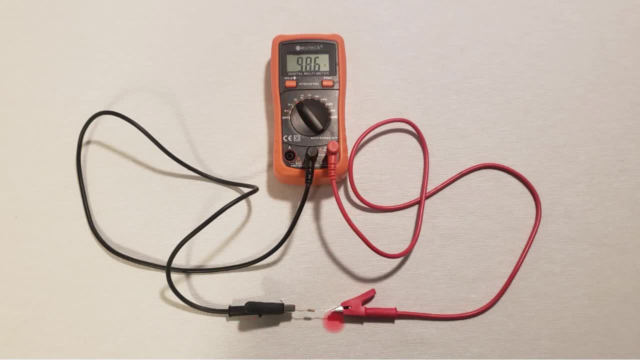 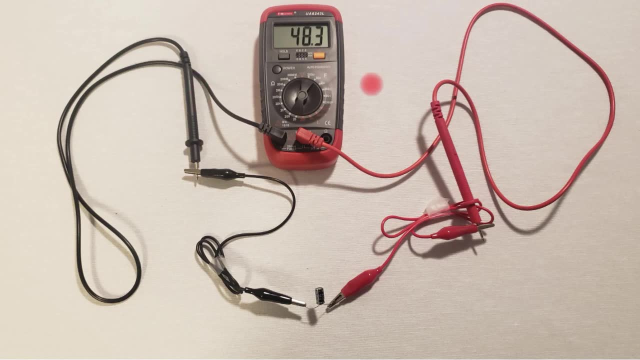 you can measure the resistance of a resistor. Just connect the test leads across it and put the setting at the ohm symbol, and you should be fine. Now, this is a completely different multimeter. So I have the black test lead connected to the left side, because that's how this type of 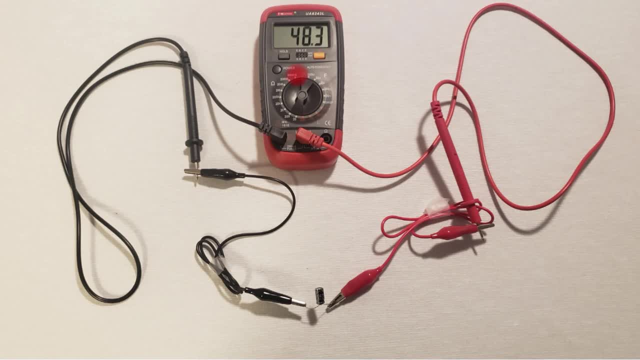 multimeter should be connected And looking at the functions here you can see that there's different values for resistance And here we have the values for capacitance, measured in like microfarads or nanofarads. HFE is for the transistor, if you want to measure the amplification.